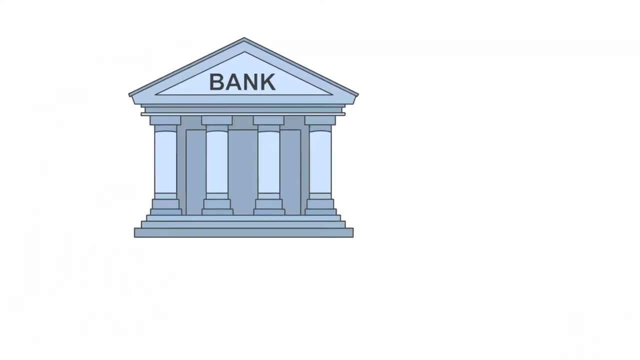 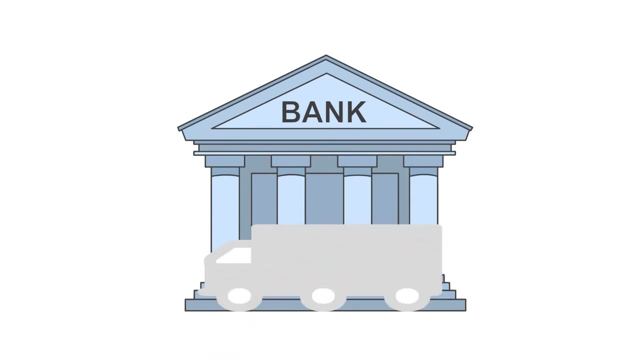 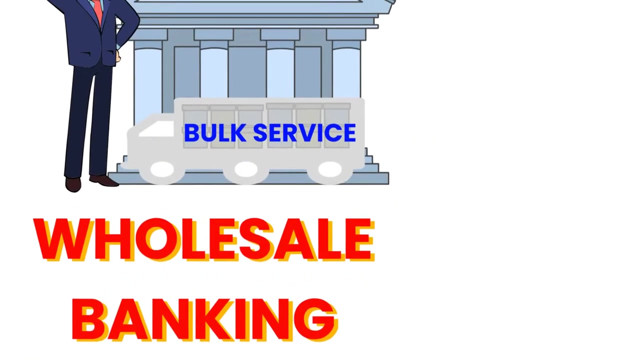 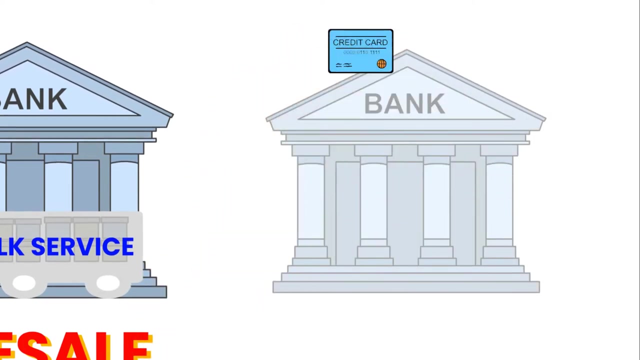 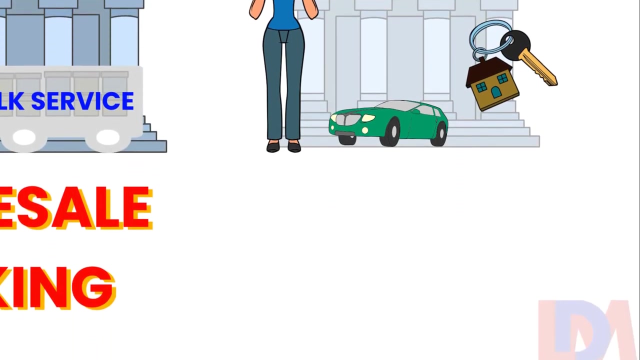 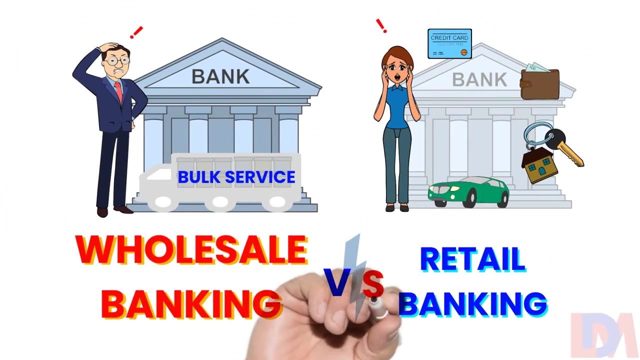 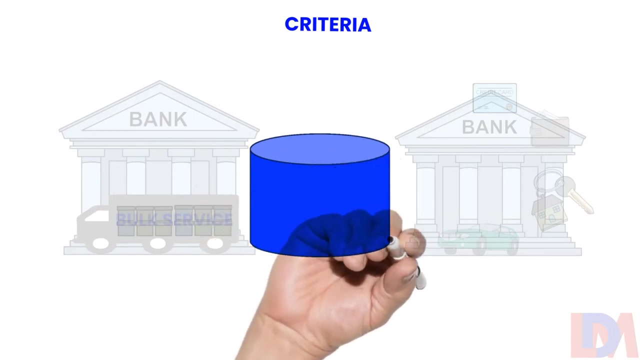 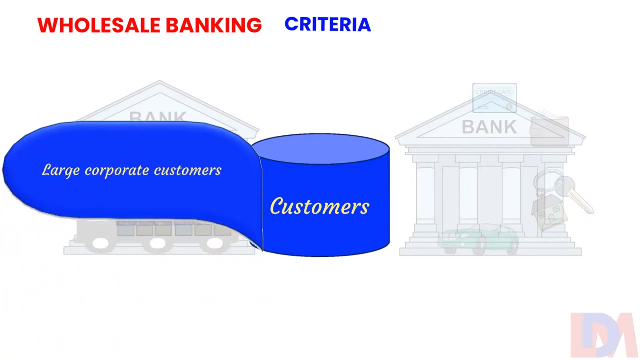 Thank you for watching. Thank you for watching. Wholesale banking refers to dealing with large corporate customers, often multinational companies, governments or government enterprises. On the other hand, retail banking refers to the mobilization of deposits, mainly from individuals, and lending to small business and in retail loan markets. 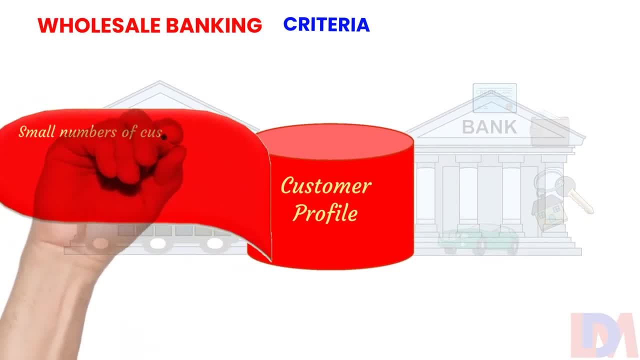 Wholesale banks usually deal with small numbers of people. Wholesale banks usually deal with small numbers of customers with large-valued transaction. They mobilize the funds from and lend funds to the business undertakings. It includes the transactions which the banks conduct with each other via interbank markets separate from customers. 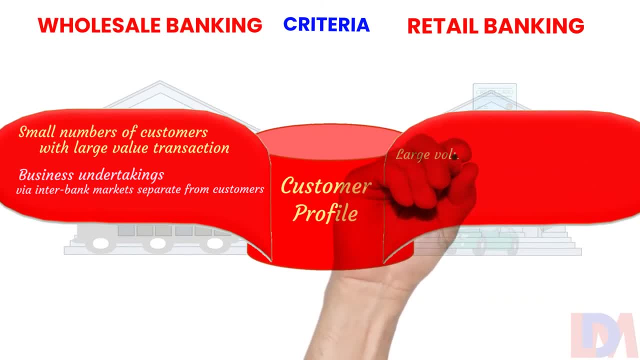 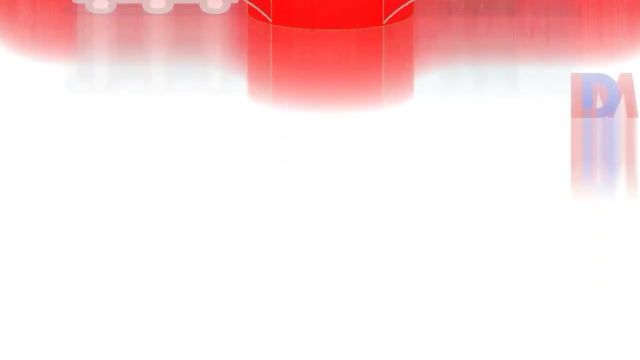 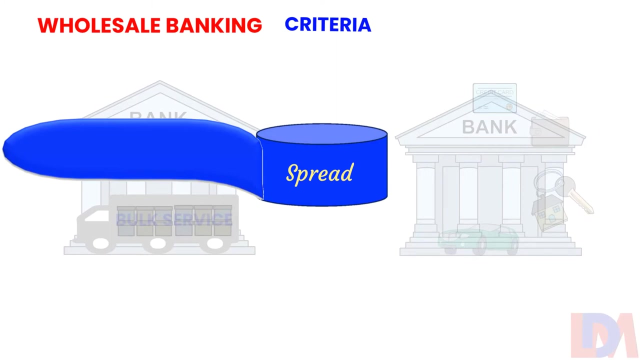 On the other hand, retail banking consists of large volume of low-value transactions. Retail banking liabilities are mostly related to various types of deposits accounts and the loan portfolio is dominated by the consumer liabilities loans. In wholesale banking, large size of deposits and loans from few customers result. 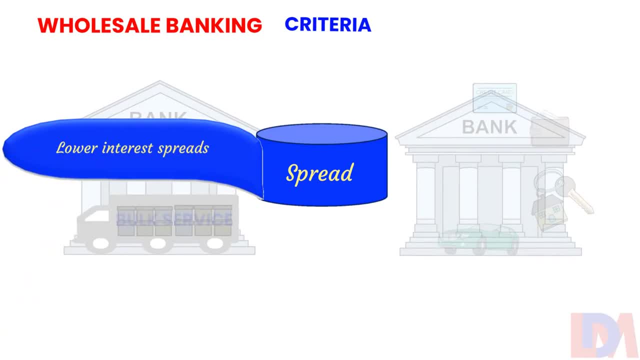 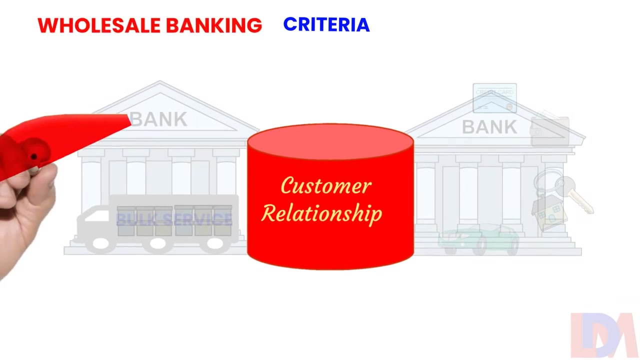 in low cost of processing, which encourages bank to have lower spreads. On the other hand, as retail banking deals with large number of customers with low value of transactions, processing cost becomes higher. Therefore, higher interest spread is maintained in retail banking transactions. Wholesale banking requires high level of customer relationship.